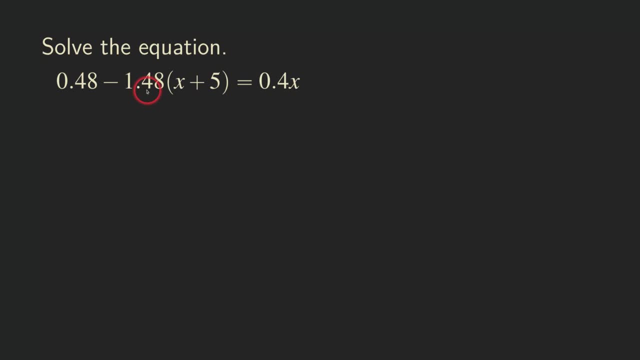 And, as you can see here, we have two digits on the right side of this dot, And then now, if you look at this number right here, this is 0.4.. For 0.4, we only have one decimal place right here, And then you may say what. 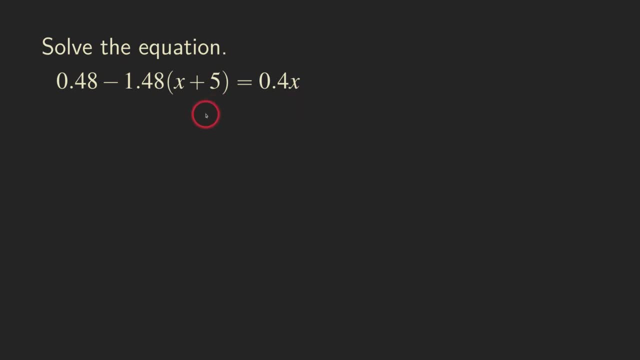 numbers. we multiply in this case because we're getting different decimal places, right. So the way to do it is that we just determine by looking at the number with the most decimal places. In this case has two decimal places. that has two decimal places and this number has one decimal place. 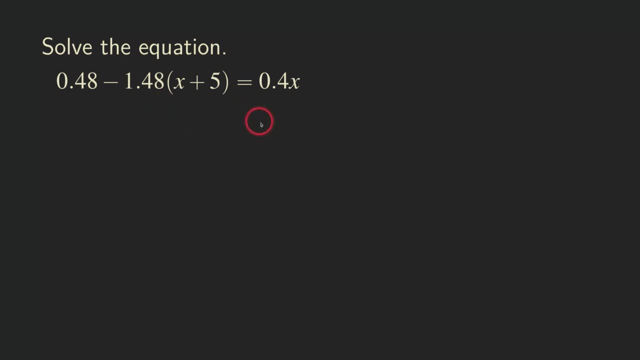 And then we are going to use the numbers with two decimal places to determine what we need to multiply. So in general, if we have two decimal places, then we need to multiply by 100 to get rid of the decimals. So what are we doing here? we are going to multiply the whole equation. 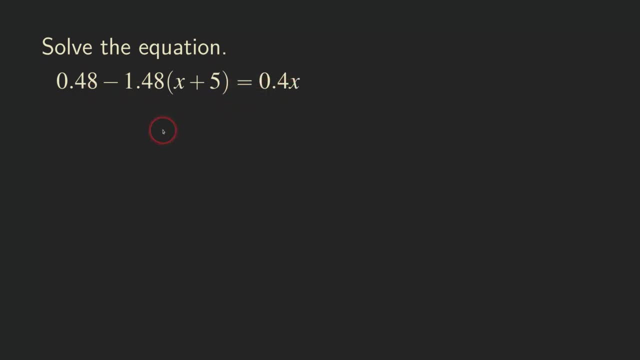 by 100.. Yeah, So let's just copy down the whole equation here. then we are going to get 0.48.. And then we need to multiply by a number, right? So let's do that. What is that number? 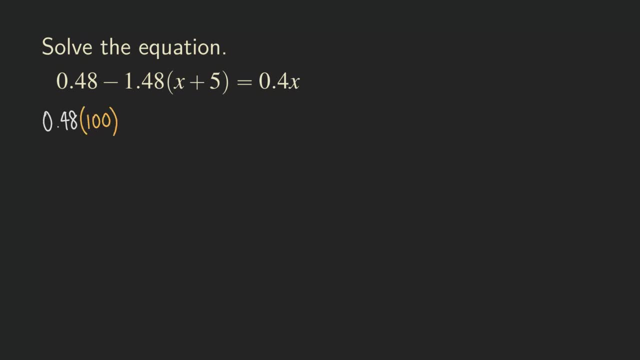 that it's going to be 100. So let me highlight the number right here. So we multiply by 100. And then next we are going to get negative 1.48. And then x plus five. then what do we need to multiply here? we need to multiply by 100. And then now what about the 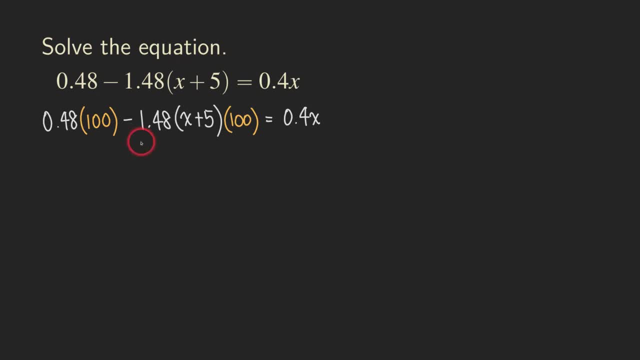 on the right hand side. Basically, once we have decided that we are going to multiply the whole equation by 100, then doesn't matter how many decimal places that you have for this one, even though it has only one decimal place, you still need to multiply by 100. So we are going 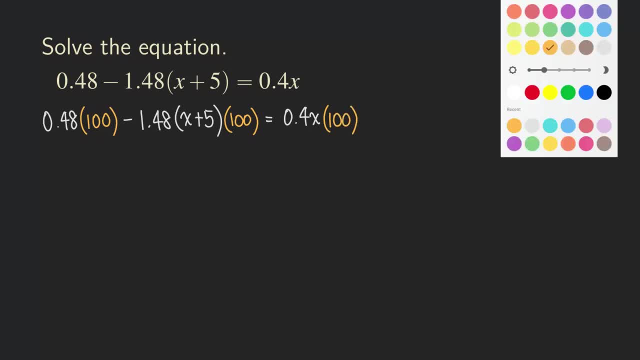 to get 100 right here. Okay, so now what are we going to do? this number, point four, eight times 100, that actually will turn in to 48. Because when you multiply a number by 100, you are going to move the decimal. 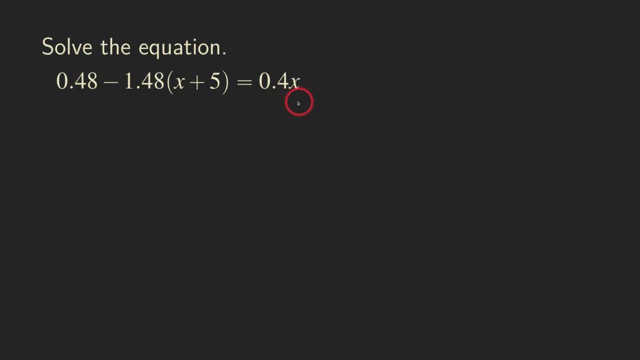 what numbers do we multiply in this case? Because we are getting different decimal places, right. So the way to do it is that we just we determine by looking at the number with the most decimal places, In this case that has two decimal places, that has two decimal places and this number has one decimal place. 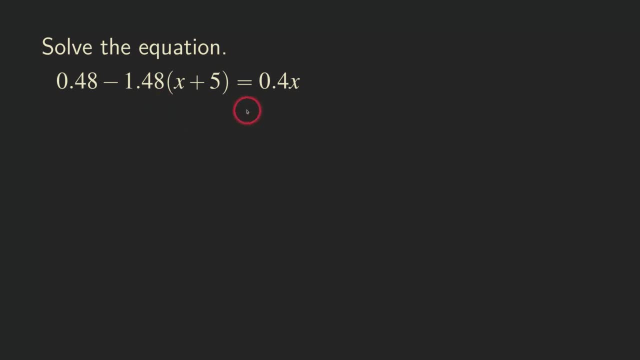 And then we are going to use the numbers with two decimal places to determine what we need to multiply. So in general, if we have two decimal places, then we need to multiply by 100 to get rid of the decimals. So what are we doing here? we are going to multiply the whole equation. 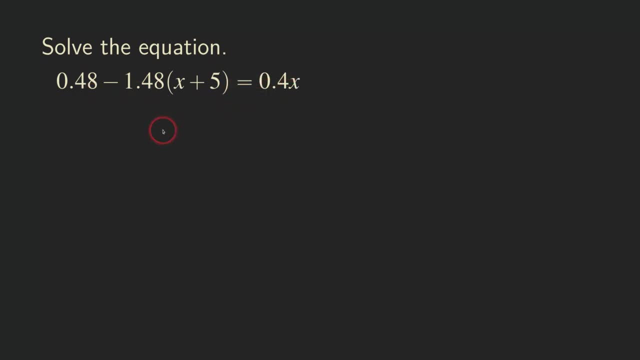 by 100.. Yeah, So let's just copy down the whole equation here. then we are going to get 0.48.. And then we need to multiply by a number, right? So let's do that. What is that number That it's. 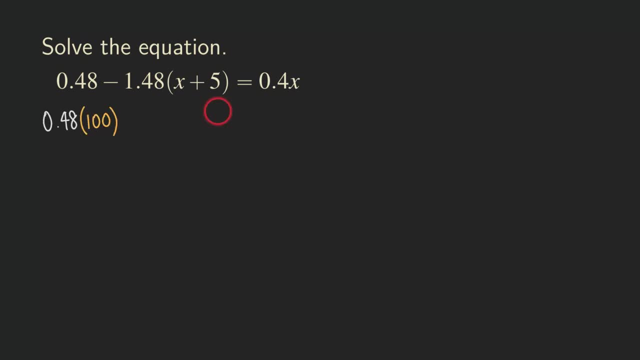 going to be 100. So let me highlight the number right here. So we multiply by 100. And then next we are going to get negative 1.48.. And then x plus five. Then what do we need to multiply here? we need to multiply by 100. 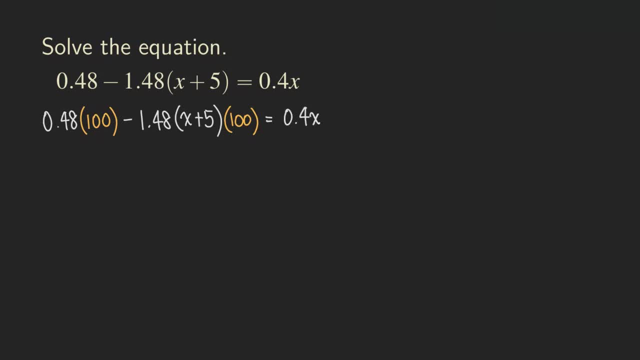 Then now, what about the equation on the right hand side? Basically, once we have decided that we are going to multiply the whole equation by 100, then it doesn't matter how many decimal places that you have for this one, even though it has only 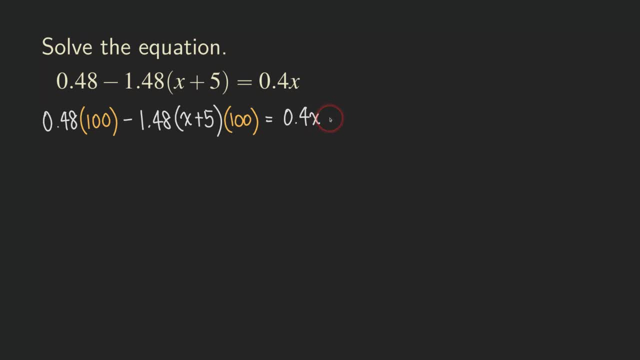 one decimal place, you still need to multiply by 100. So we are going to get 100 right here. Okay, so now what are we going to do? This number, point four, eight times 100, that actually will turn into 48. Because when you multiply a number by 100, you are going to move the decimal to the 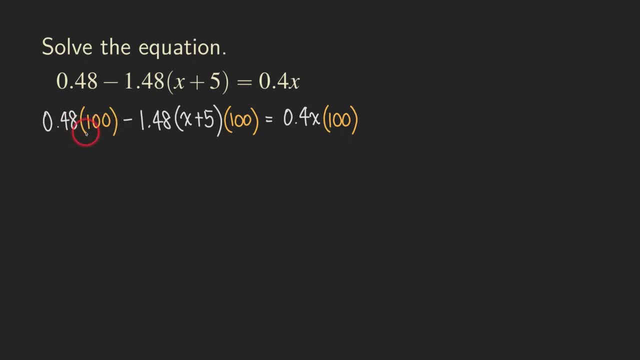 right two times, because there are two zeros in this 100 right here. right? So you're going to make this number 100 times itself. So you are going to get one, and then two, So you're going to get 48 for this number. So we have 48 right here, And then now the minus sign. 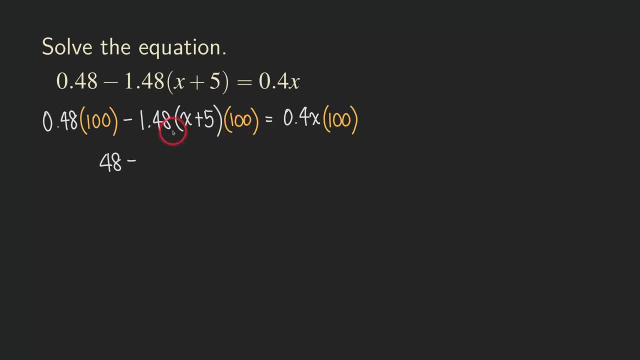 Now we take the 1.48 and times 100. And we are going to move two decimal places. So we are going to get one and two, So we are going to get 148.. And then you may say: what about the stuff that's? 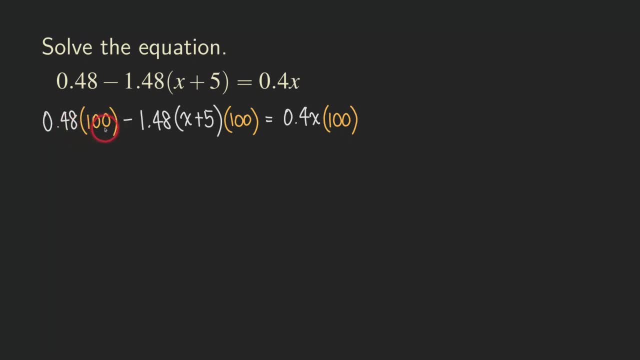 to the right two times, because there are two zeros in this 100 right here. right? so you're going to make this number 100 times itself. so you are going to get one, and then two, so you're going to get 48 for this number. So we have 48 right here, And then now the minus sign. 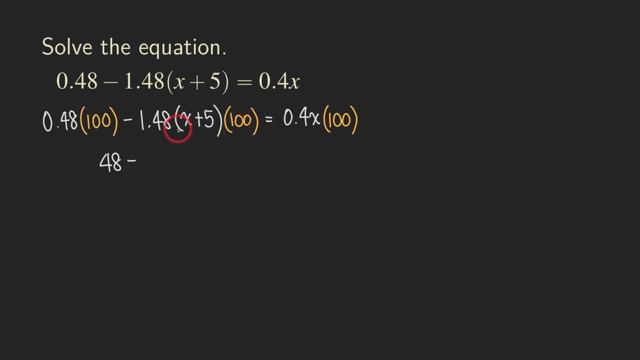 Now we take the 1.48 and times 100. And we are going to move two decimal places. So we are going to get one and two, so we are going to get 148.. And then you may say: what about the stuff that's? 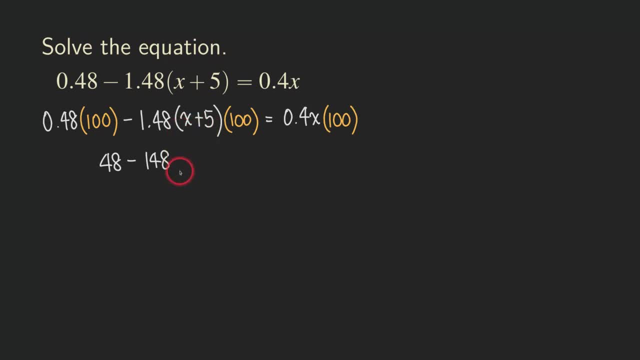 inside the parentheses. we are not going to touch them, So we are just going to copy. all you need to do is to turn this decimal into this whole number right here, by multiplying by whatever number that we need to multiply. In this case is the 100.. And we are not. 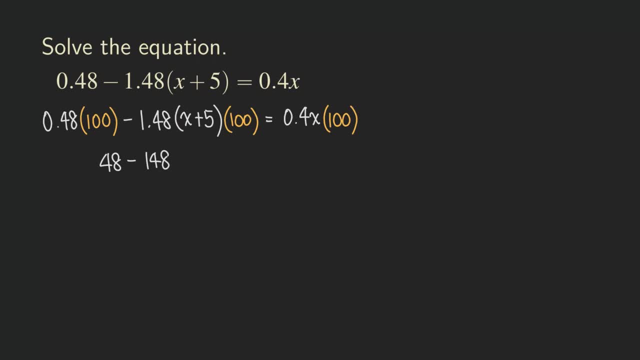 going to worry about anything that's inside the parentheses yet. Okay, so just copy. And then we are going to get equal, right. And then what do we get here? this is point four, and then times 100.. Now, if you put four right here, that will not be correct, Because remember. 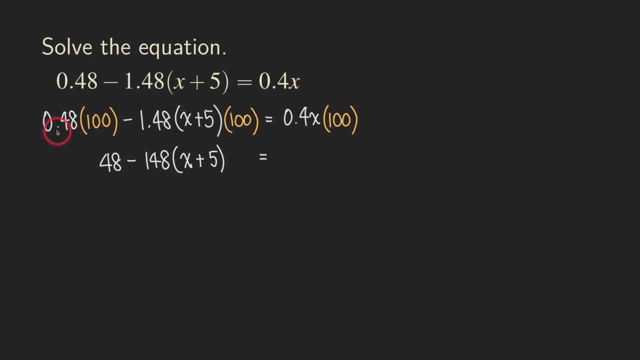 that I mentioned right here when I did the multiplication with a point four, eight times 100, we move the decimal dot two places to the right right Now, if you just imagine that you are going to move this point four, I mean this point, this decimal point two places to the right. 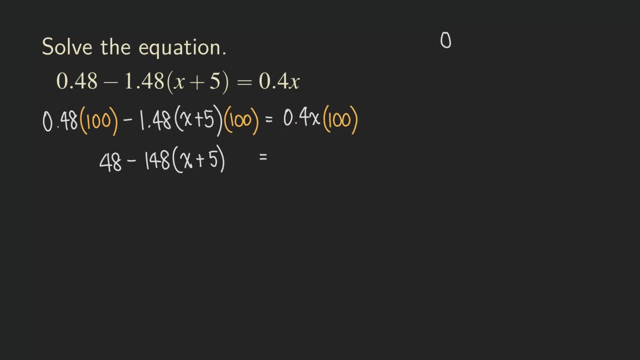 and then it's going to look like this: So we have point four. So let's do some scratch work on the side here. If you move two places, then it's going to look like this: So that's one, Okay, And then you need to do one more. 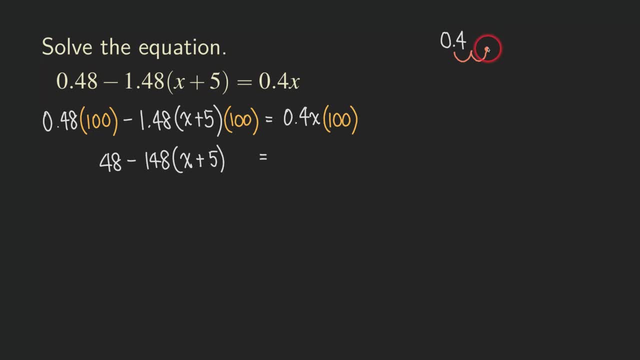 So now that's your new decimal dot. And then and then now there was no numbers right here. what do you need to do? you need to actually place a zero to hold the place. So you are going to get zero right here. So now, what does that number become? And actually remember that now the 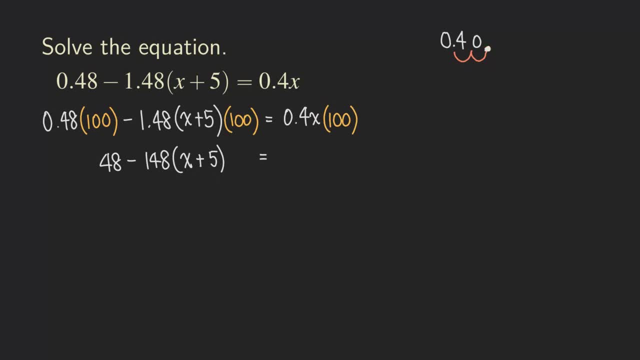 new decimal point is right here, So it's right here. So what does that mean? That means that number actually is 40.. Okay, And then don't forget that there was still an x in there, So we just copy down the x. 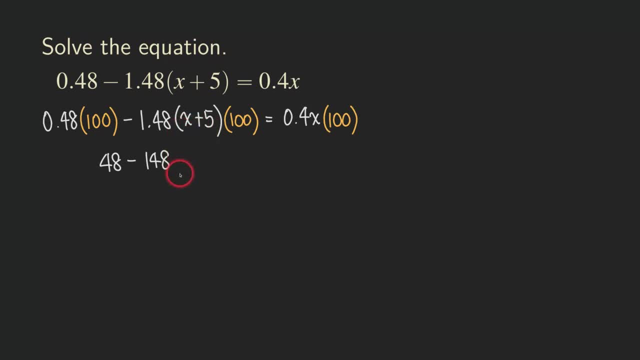 inside the parentheses. we are not going to touch them, So we are just going to copy. all you need to do is to turn this decimal into this whole number right here, by multiplying by whatever number that we need to multiply. in this case is the 100.. And we are not going to worry. 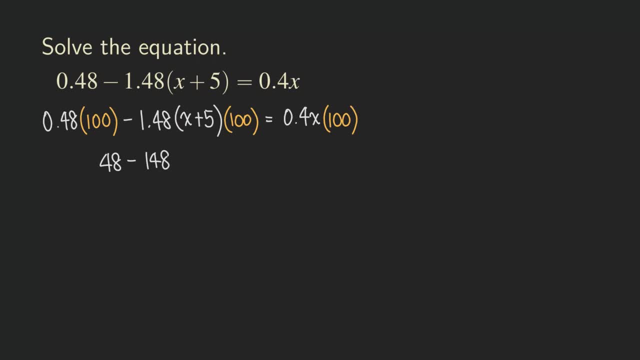 about anything that's inside the parentheses yet. Okay, so just copy. And then we are going to get equal, right. And then what do we get here? this is point four, and then times 100.. Now, if you put four right here, that will not be correct. So we are going to put four right here and then times. 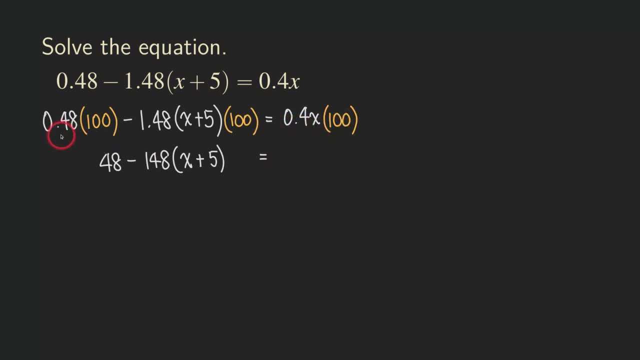 correct Because remember that I mentioned right here when I did the multiplication with a point four, eight times 100, we move the decimal dot two places to the right right Now, if you just imagine that you are going to move this point four, I mean this point, this decimal point. 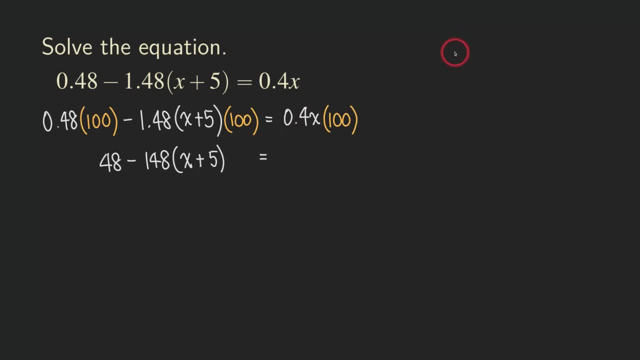 two places to the right, and then it's going to look like this: So we have point four. So let's do some scratch work on the side here. If you move two places, then it's going to look like this: So that's one, Okay, and then you need to do one more. So now that's your new. 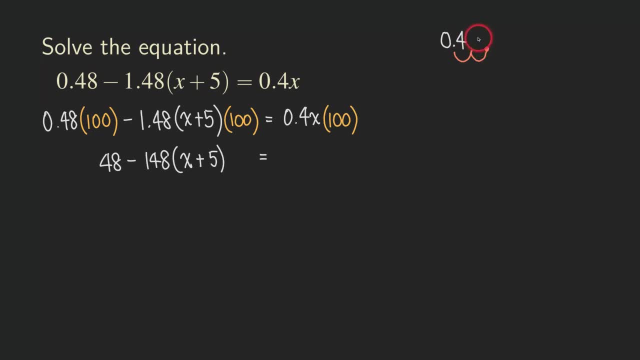 decimal dot And then-and then. now there was no numbers right here. What do you need to do? you need to actually place a zero to hold the place. So you are going to get zero right here. So now, what does that number become? And actually remember that. now the new decimal point. 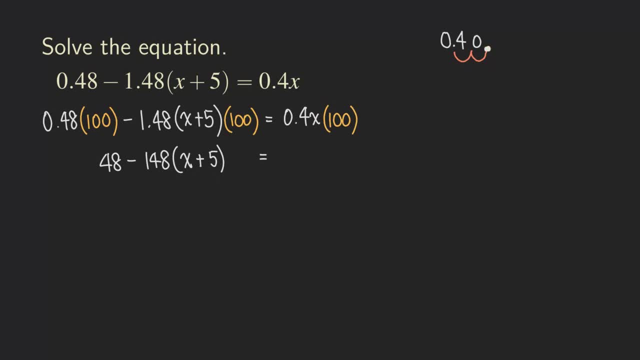 is right here. So it's right here. So what does that mean? That means that number actually is 40.. Okay, And then don't forget that there was still an x in there, So we just copy down the x. we didn't do anything to the x, So just just copy, Okay. so now we get this equation And we are. 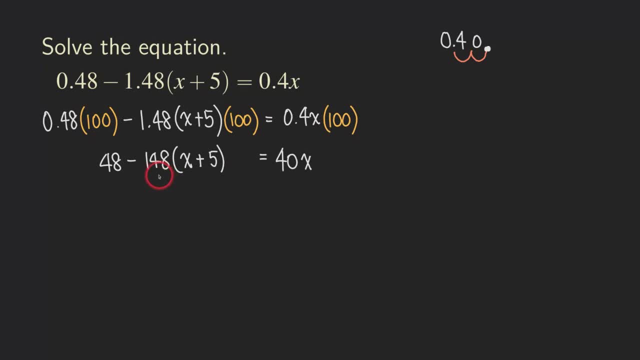 seeing a pair of parentheses right here. So the first thing that we need to do is to just multiply this negative. I mean, distribute this negative 148 to the x and to the five. then let's do that, So we distribute this to the x and then distribute to the five. So we are going to get what? 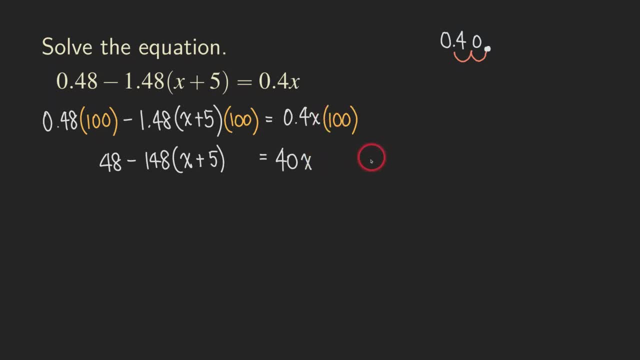 we didn't do anything to the x, So just just copy. Okay, so now we get this equation And we are seeing a pair of parentheses right here. So the first thing that we need to do is to just multiply this negative, I mean, distribute this negative 148 to the x and to the five. then let's do that. 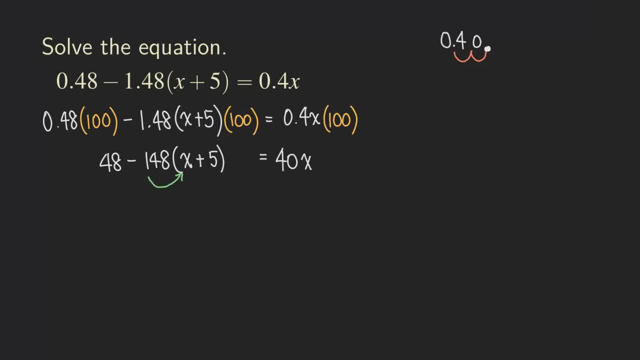 So we distribute this to the x and then distribute to the five, So we are going to get what? Well, the 48, we just copy it down, And then we are going to get negative 148. And then the x, And 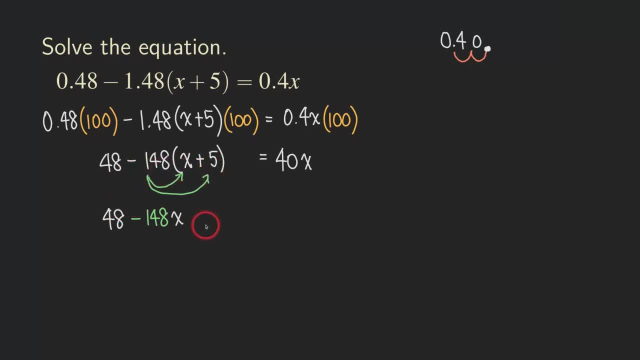 then you may say: what about the negative 148 times the five right? So we can do the calculation on the side right. here We can do the calculation like 148.. So just some more scratch work on the side 148.. And then times the: 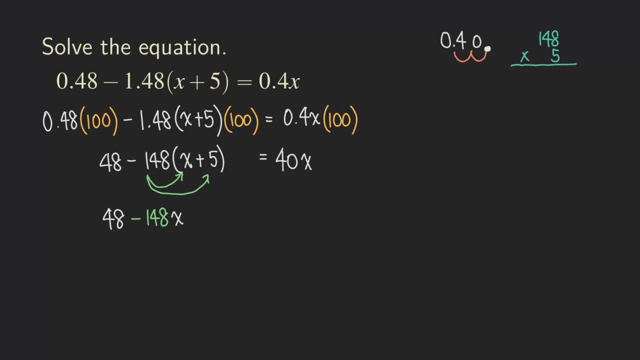 five. we can do a long multiplication. So five times eight is 40.. And then four times five is 2024.. Right, So we have 24.. And then one times five is five plus two is going to be seven. Okay, so that's actually the 740.. Right, And now it's negative. 148 times positive. So we 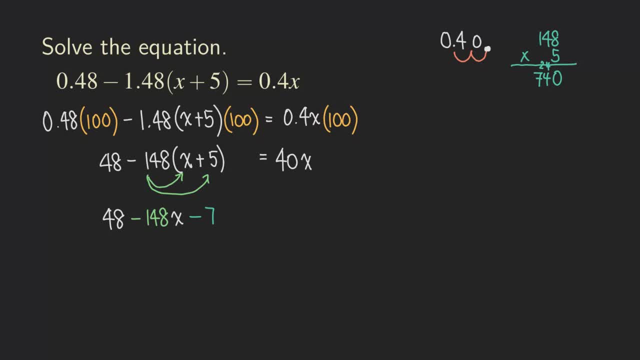 are going to get a negative number right here, So it will be negative four negative 740.. And then we didn't touch anything on the right hand side here, So we are going to get 40x. Okay, so if it turns out we can combine- we should really combine them right now- So it's the 48 minus the. 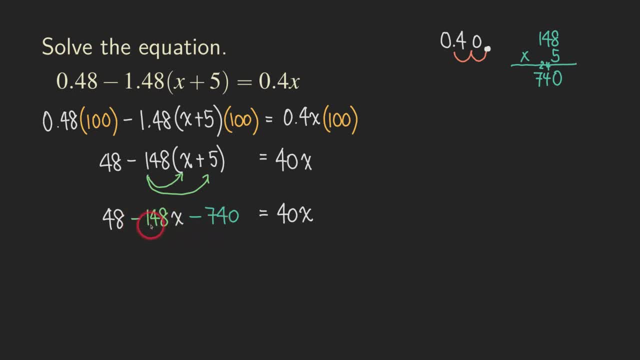 740, we can combine them. then we are not going to do anything to this negative 148x. So I'm just going to copy it down first. Then you may say: what about the 48 minus 740,? then we are going to. 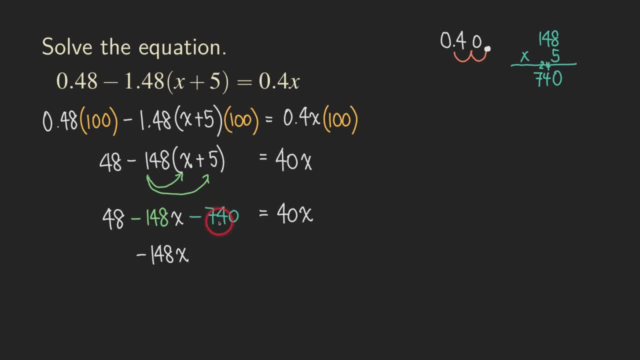 get what it's going to be: a negative number, because this negative it's negative: 740, plus the 48,. right, so we would get it When we have different signs. we got to do subtraction And so we are going to get minus. 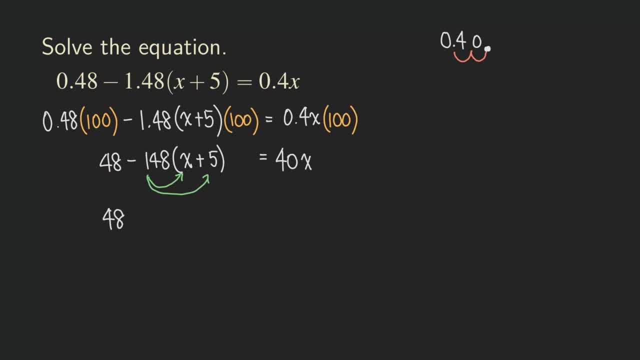 Well, the 48, we just copy it down And then we are going to get negative 148.. And then the x. And then you may say: what about the x? And then you may say what about the x? And then you may say: 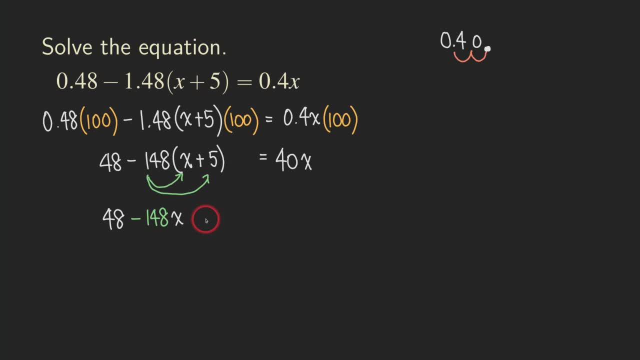 the negative 148 times the five, right, so we can do the calculation on the side right. here we can do the calculation like 148. so just some more scratch work on the side 148 and then times the five we can do a long multiplication. so 5 times 8 is 40, and then 4 times 5 is 2024, right? 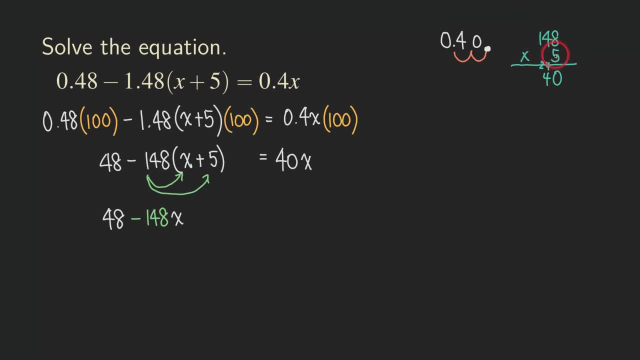 so we have 24, and then 1 times 5 is 5 plus 2 is going to be 7.. okay, so that's actually the 740, right, and now it's negative 148 times positive. so we are going to get a negative number right here, so it will be. 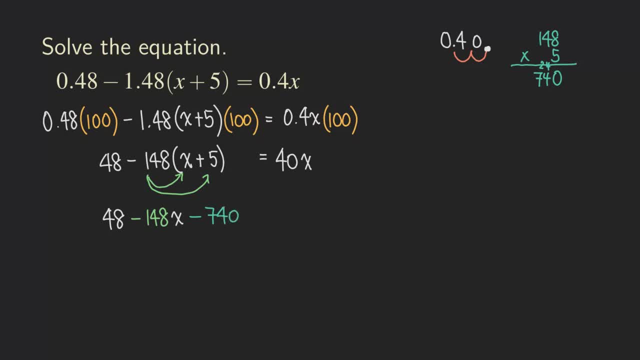 negative 4 negative 740, and then we didn't touch anything on the right hand side here. so we are going to get 40x. okay, so if they're like turns out, we can combine. we should really combine them right now. so it's the 48 minus the 740. we can combine them. then we are not going to do anything. 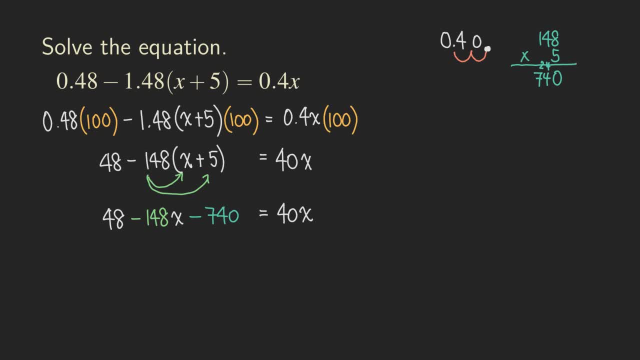 to this negative 148 x. so i'm just going to copy it down first. then you may say: what about the 48 minus a 740? then we are going to get what? it's going to be a negative number, because this negative, um, it's negative 740 plus the 48, right? so 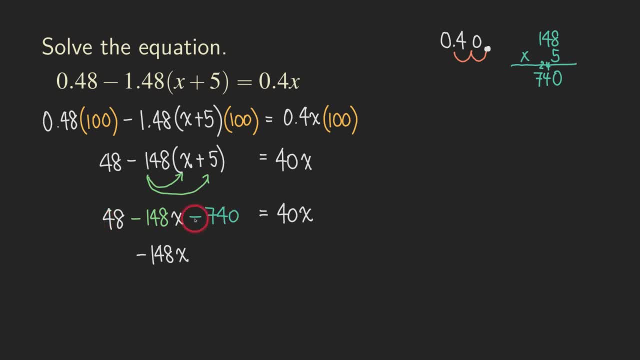 we we got when we have different signs. we got to do subtraction and so we are going to get minus. okay, 740 minus 48, so we are going to get negative 600, and then we have 92, and then we have the 40x on the right hand side of the equation. 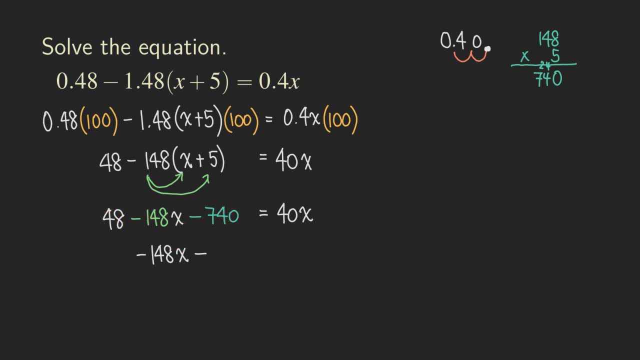 okay, 740 minus 48. So we are going to get negative 600. And then we have 92. And then we have the 40x on the right hand side of the equation. Okay, so next step is that we want to subtract 40x from both sides of the equation because we can get 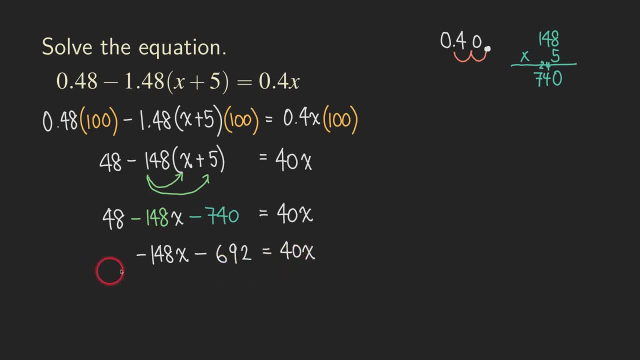 rid of this 40x so that we can get all the x turns on the left side of the equation, Or actually we can move this one to that side right, So we can actually just add 148x to both sides of the. 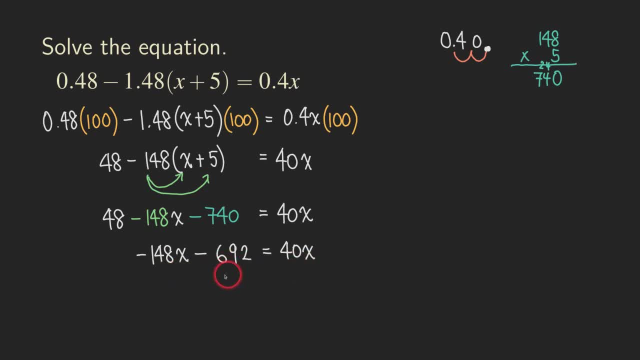 equation, then we can still get all the x turns on the left side and then get all the non-x turns on the left side. So let's do that, So we can add 148x, So 148x, and you see that. 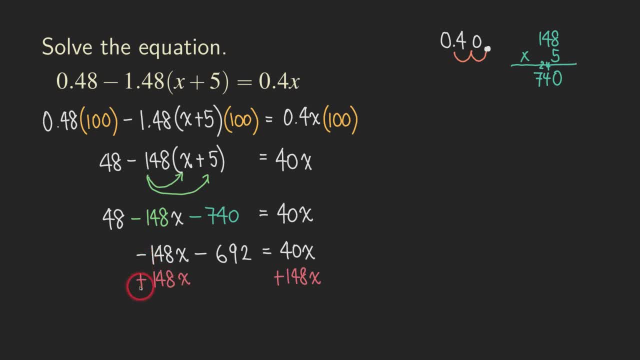 those two terms, they will get cancelled because we have one positive 148, and the other one is a negative 148.. So we can cancel them here completely. then you are going to get zero for that. So continuing with the calculation here. 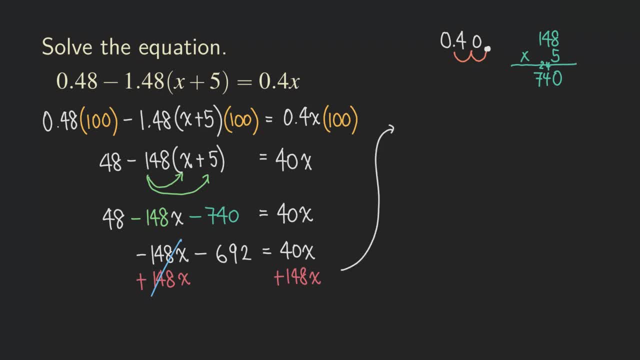 on the 148 and 148.. So we are going to multiply x, so 148x is negative 148x, So we can increase the value. So 148x here 148. So 148x times 148x is 0.. So, continuing with the calculation here, we are gonna get 0 for that. So, continuing with the calculation here, 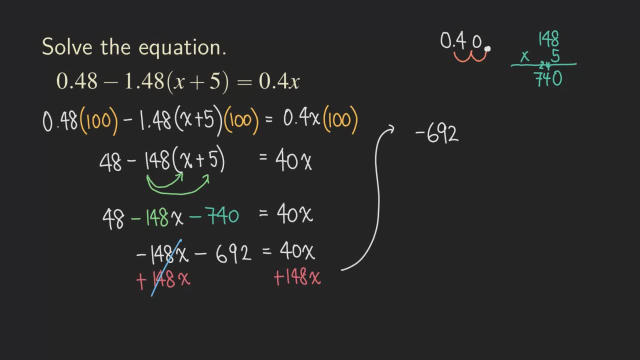 to get negative 692 on the left side of the equation. And then what about the right side of the equation? we actually need to add the 40x and the 148 x together, So we are going to get one. what is that? That's 188?. Yeah, so that's 188, right, 148 plus 40. So we get 188 x. 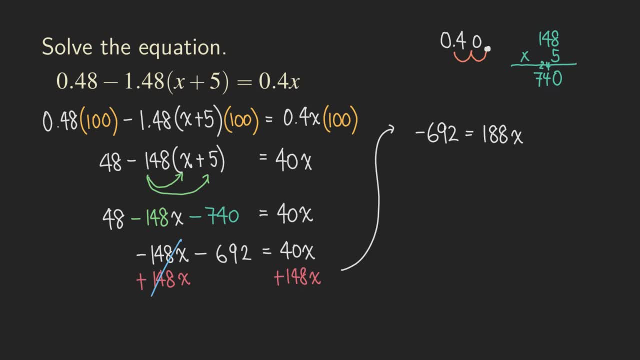 Okay, so what is the next step? The next step is to to get rid of the coefficient of the x to turn into a one. actually not getting rid of it, It's just yeah. So what are we doing? Actually, in this case, we are going to divide both sides by this number. 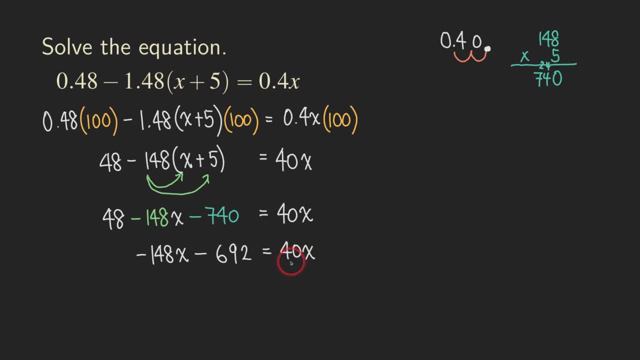 okay. so next step is that we want to subtract 40x from both sides of the equation, because we can get rid of this uh 40x, so that we can get all the x turns on the left side of the equation, or actually we can do, we can move this one to that side right, so we can. we can actually just add 148x. 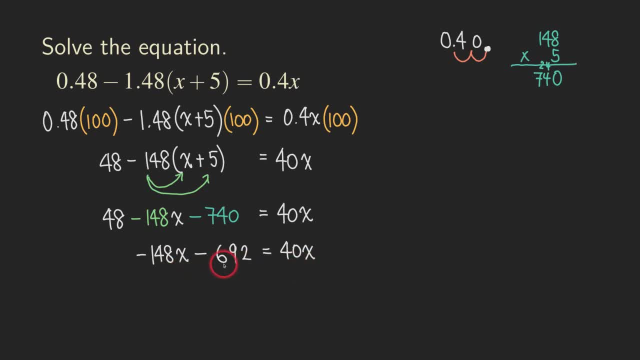 to both sides of the equation, then we can still get all the x turns on the left side and then get all the non-x turns on the left side. so let's do that, so we can add 148x, so 148x. see that those two turns, they will get canceled because we have 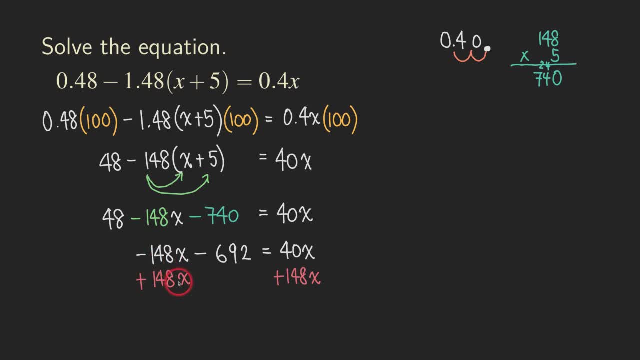 one positive 148 and the other one is negative 148. so we cancel them here completely. then you are going to get zero for that. so, continuing with the calculation here on, we are going to get negative uh 692 on the left side of the equation. then what about the right side of the equation? we actually need to add the 40x and the 140x. 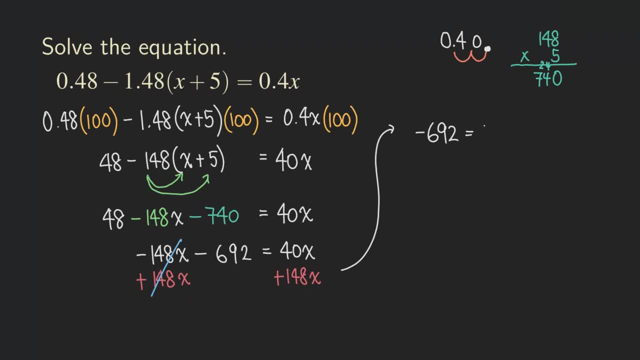 148x together. So we are going to get 1,. what is that? That's 188.. Yeah, so that's 188, right, 148 plus 40. So we get 188x. Okay, so what is the next step? The next step is to get rid of the coefficient of the x. 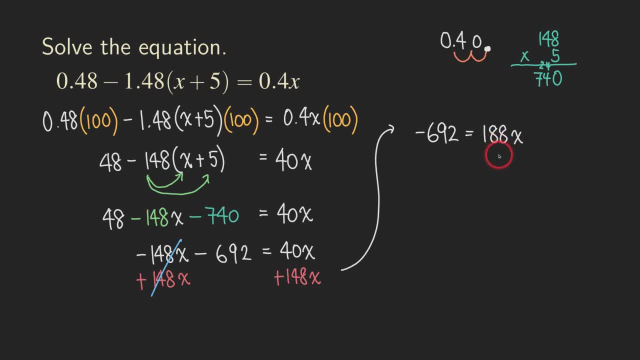 to turn it into a 1.. Actually not getting rid of it, it's just yeah. So what are we doing actually? in this case, We are going to divide both sides by this number in front of the x, which is 188.. 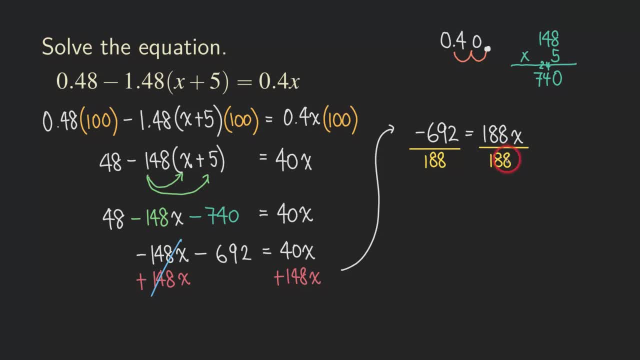 Okay, So you know that the 188, when you divide them you are going to get 1, right? So you're going to just get 1 here. so the x is already isolated, This one. we basically will say that this is the. 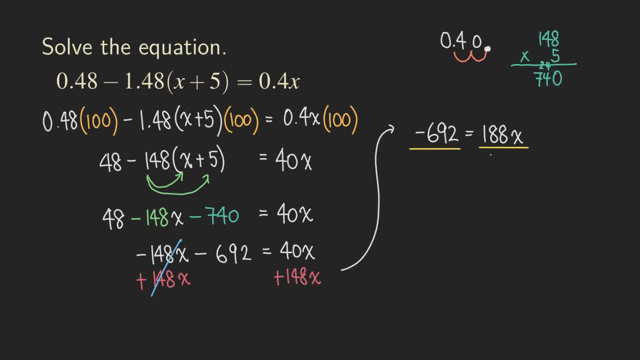 in front of the x, Which is 188.. Okay, so you know that the 188 and the 188, when you divide them you're going to get one right. so you're going to get. just get one here. So the x is already isolated. 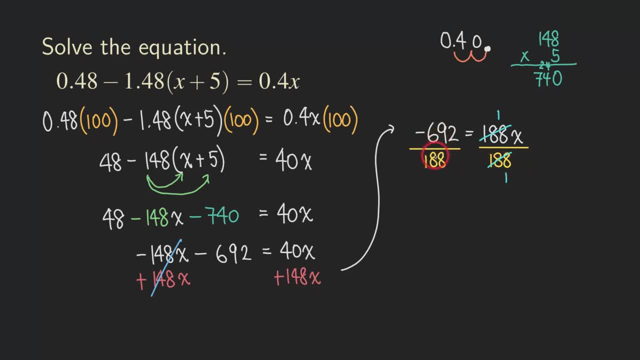 This one. we basically will say that this is the answer, but then we can actually Reduce the fraction. to make it more simplified. In this case we can try dividing by four, because they're both even numbers And the last two digits actually tell us that four will go into both numbers. 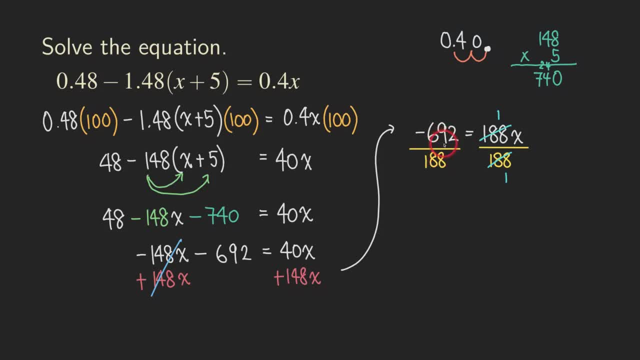 Maybe the larger numbers will go in there, but then we should really just check the five by four and then just keep reducing it right? So let's divide by four for both the the 692 and then the 188.. So let's do that. 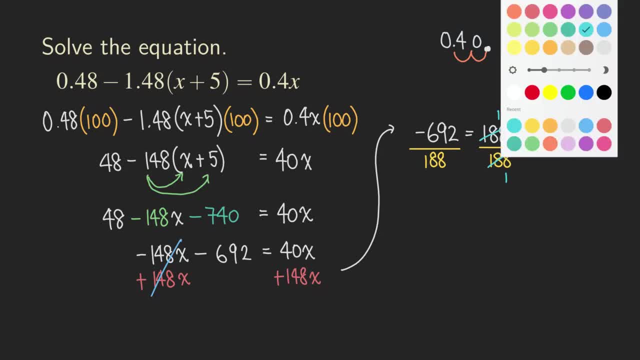 So if you divide by four here, Okay, so let me see what color that I can use right here. So maybe I can use the this color right here. So divide by four, Okay. So basically we are doing 692,, right, 692, and then we are dividing by four. 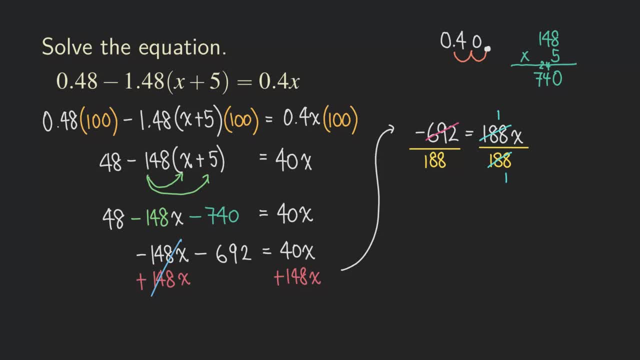 So 692 divided by four, That's going to be 173, okay, and then the 188, and we want to divide that by 4. we are going to get divide by 4, that's 4, then you're gonna get to 28 and then 7, right, so 47 and can. 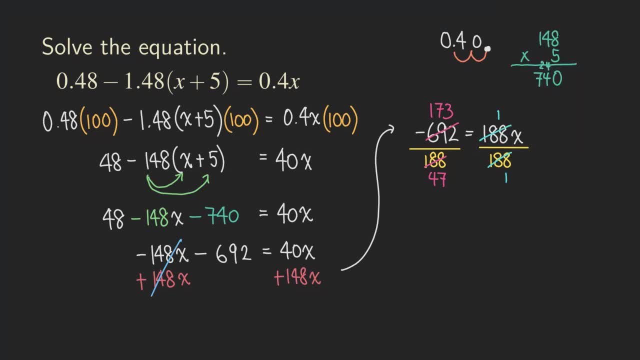 we continue to reduce that. no more right. so we are going to have my answer to be X on this side. right, because we have 1 over 1 times X, so we get X. what about the left side? I mean, yeah, the left side. we have negative. what? 173 over the 47. 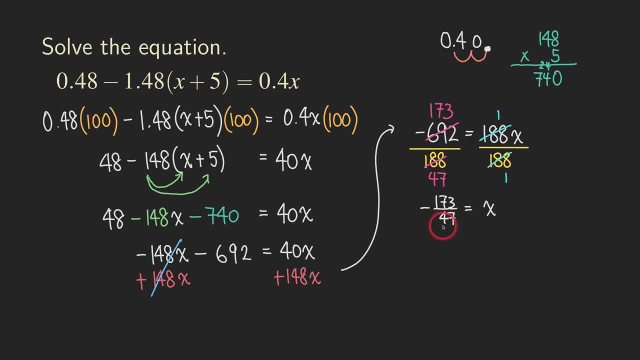 and then if you want to have the X on the left side, so we say that X is equal to a negative 173 over 47, and then we are finished with this problem. you can use your calculator and turn this into a decimal, but it's again, it's just unnecessary, right? so we 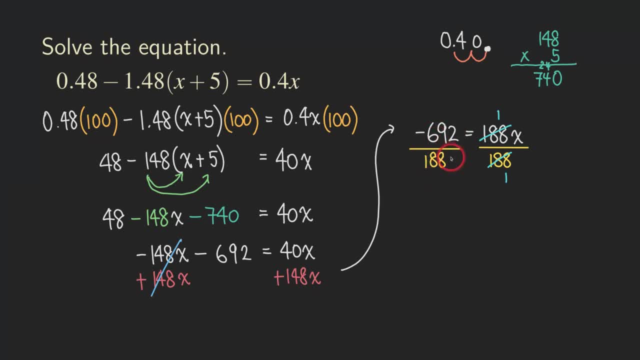 answer, but then we can actually reduce the fraction to make it more simplified. In this case, we can try dividing by 4, because they're both even numbers and the last two digits actually tell us that 4 is the answer. So we can actually reduce the fraction to make it more simplified. 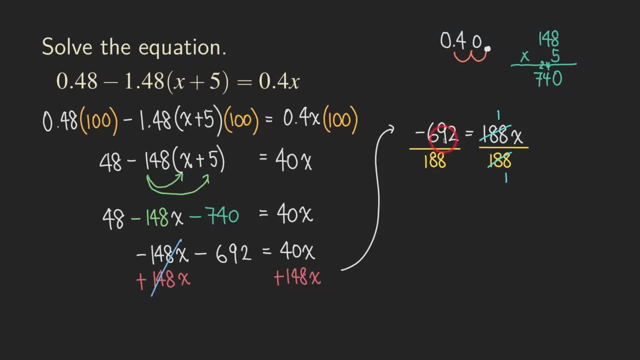 Maybe the larger numbers will go in there, but then we should really just check the 5x4 and then just keep reducing it, right? So let's divide by 4 for both the 692 and then the 188.. So let's do that. So if you divide by 4 here, Okay, so let me see what color that I can use. 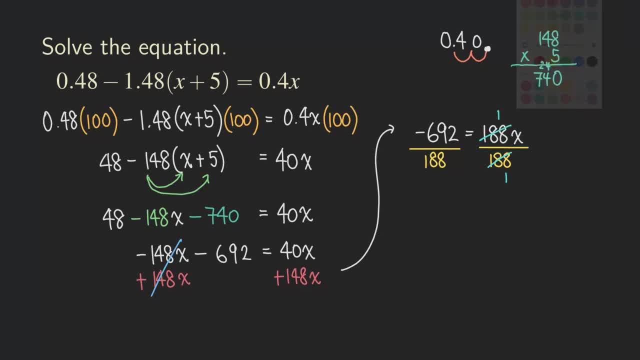 right here, So maybe I can use this color right here. So divide by 4.. Okay, so basically we're doing 692, right, 692, and then we are dividing by 4.. So 692 divided by 4, that's going to be 173. Okay, And then the 188, and we want to divide that by 4, we are going to. 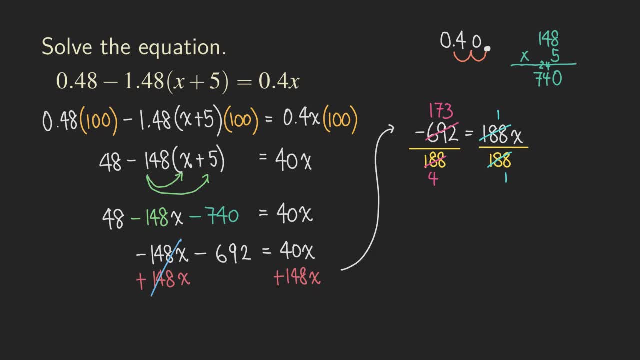 divide by 4,, that's 4.. Then you're going to get to 24.. And then 7,, right? So 47. And can we continue to reduce that? No more, right? So we are going to have my answer to be: 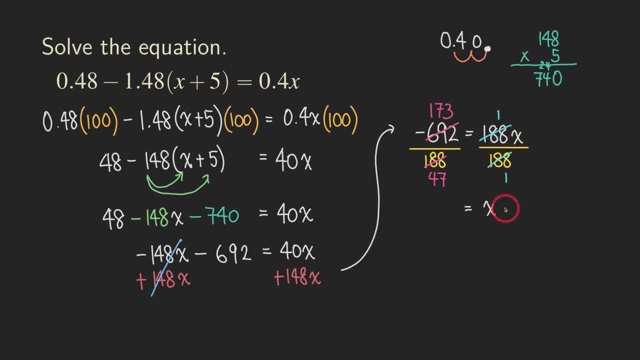 x on this side, right, Because we have 1 over 1 times x, so we get x. What about the left side? I mean, yeah, the left side. we have negative. what? 173 over the 47. And then, if you want to, 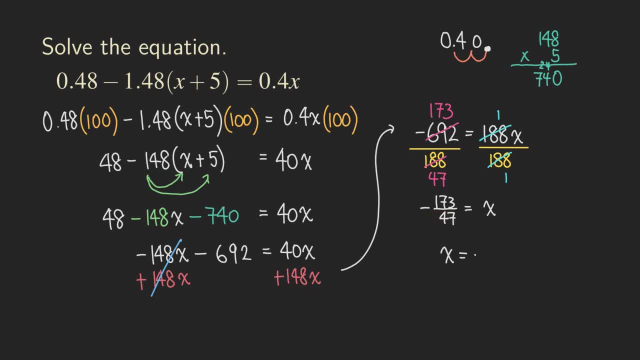 have the x on the left side. so we're going to have the x on the right side. So we're going to have the x on the left side. So we say that x is equal to negative 173 over 47. And then we are. 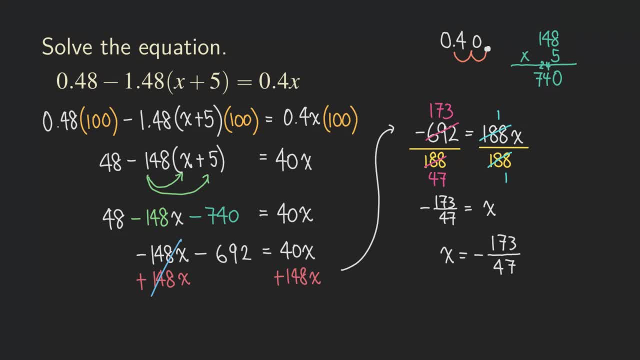 finished with this problem. You can use your calculator and turn this into a decimal, but it's again, it's just unnecessary, right? So we're going to leave the answer like this: Yeah, Okay, so that's it for this problem And thank you for watching. I will see you next time.